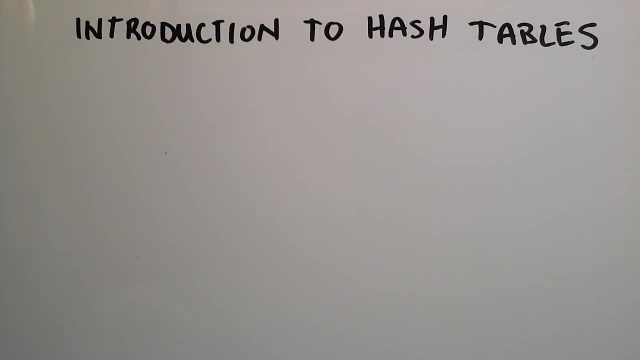 Hey everybody, this is Paul, So in this tutorial I'm going to do an introduction to hash tables. So a hash table is a data structure that is used to store information. So the information in a hash table basically has two main components. So it's going to have some sort of key and 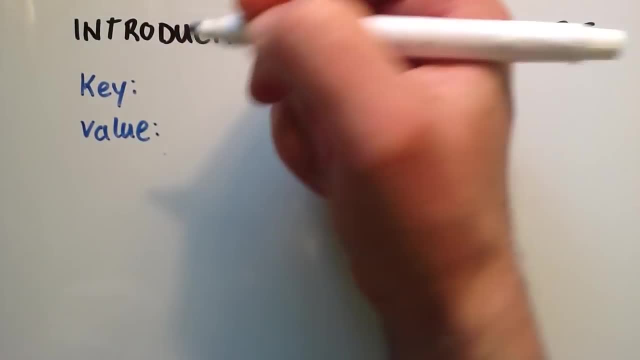 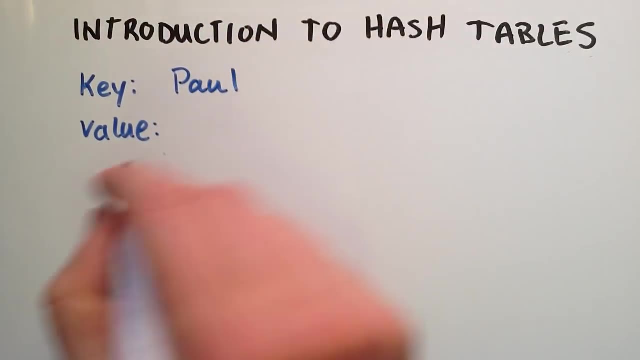 then it's going to have some sort of value or some sort of record, And so basically a key could be something like, for instance, my name And the value could be something like my phone number, So we could basically create a hash table to store a bunch of people's. 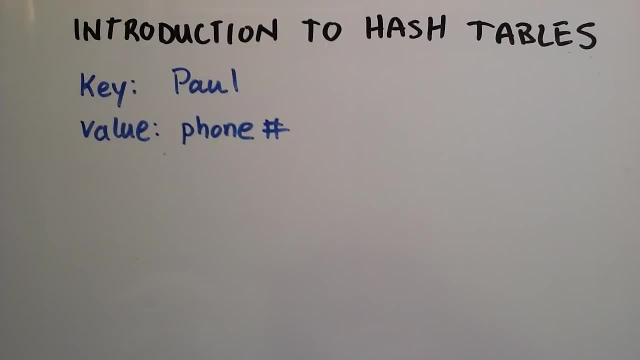 phone numbers. And so what happens is the hash table. it's a way that we can implement an associative array, And so we're basically going to map this key to this value here And at the heart of a hash table. we're basically just going to have this array structure. 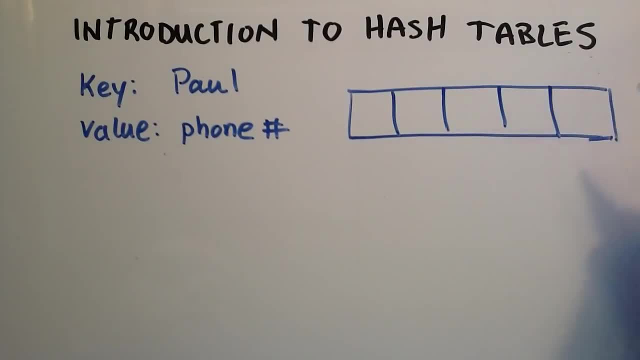 And so this has got a bunch of different array elements here And we've got index 0,, 1,, 2,, 3, and 4.. And if we were to really create a real hash table, if we were going to actually 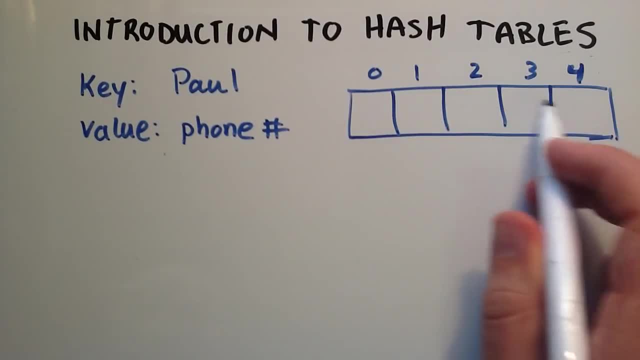 implement this in code. we're going to make our hash table be much bigger than this, But this is just kind of for illustrative purposes, So this information can fit on the whiteboard here, But in reality we would normally make hash tables much larger than this. So, anyway, 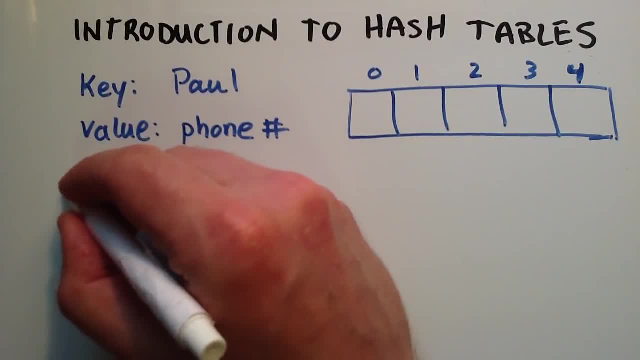 so the way this works is: we're basically going to write a hash function, And so what the hash function is going to do is it's going to look at a certain key And then it's going to evaluate that key And it's going to spit out some sort of index number And it's going 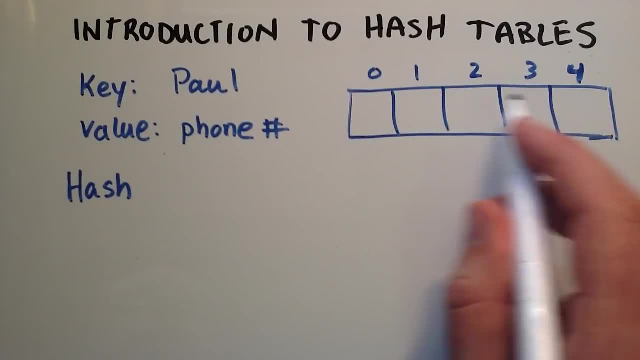 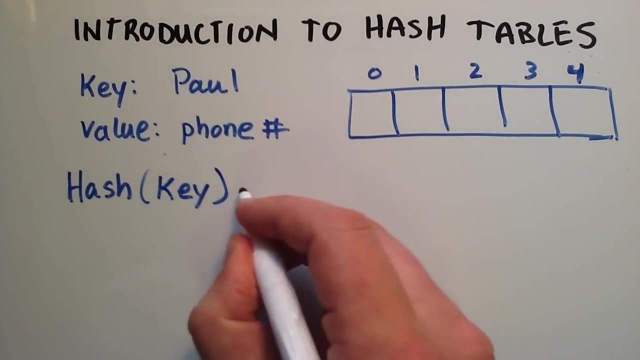 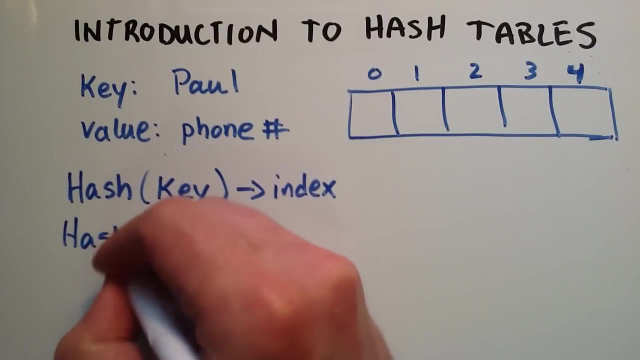 to tell us what location in the array to store this information. So, for example, we'll just go ahead and just write this out. So our hash function is going to take a key value And it's going to give us an index number. So, for example, we could do hash And then, as: 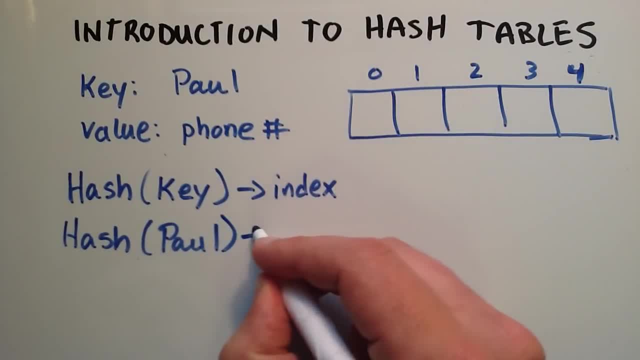 the argument. we could enter my name. My name could be the key, And then we could just say that our hash function evaluated this key And it said: OK, that should go in index 3.. And the way the hash function is written is that every time you enter that key, if 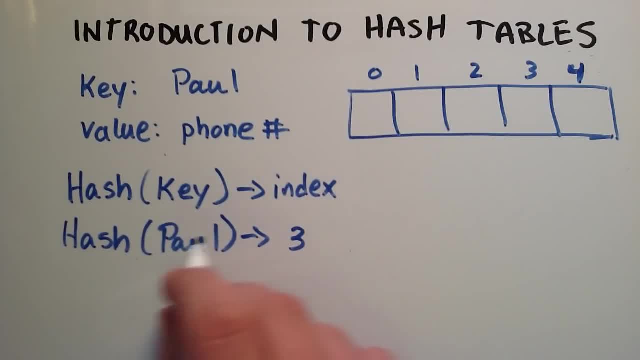 it's the same key, it's going to spit out the same index number. So every time I enter my hash function, I should get the index number of 3.. So we could just represent Paul as a circle. So we'll just go ahead and put that here. 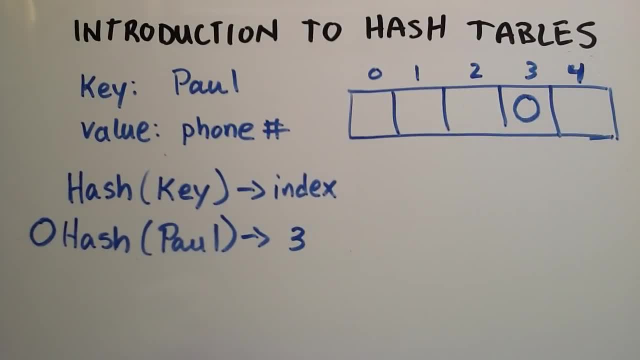 So this circle is going to represent my name and my phone number and where it is located in the hash table. So let's say that we wanted to add some other person. So what we would do is we would just put whatever that person's name is as the key. So it's going to evaluate. 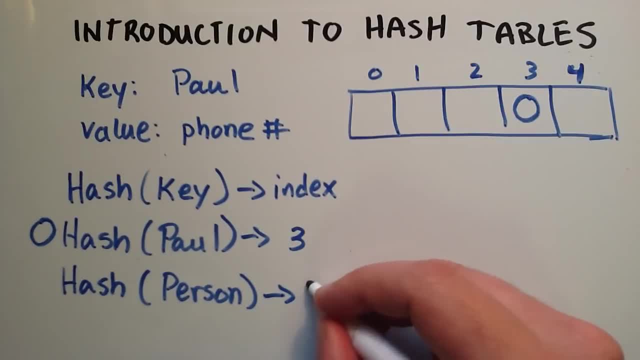 person And we'll just say that it spits out an index value of 3.. And then we'll just go ahead and put that person's name as the key. So it's going to evaluate person And we'll just say that it spits out an index value of. 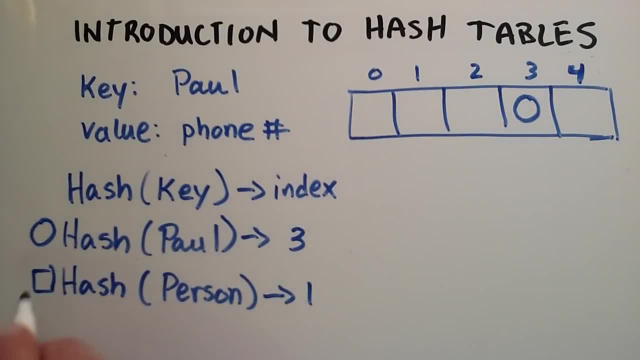 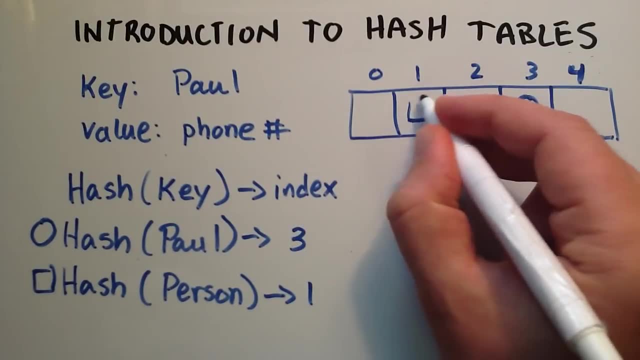 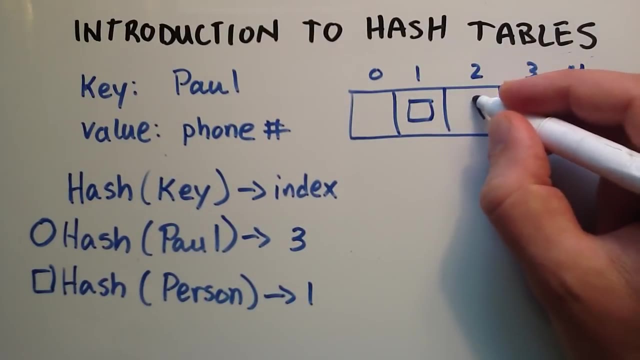 1. So person can be square, I guess. So this square will represent some other person's name and phone number And according to our hash function we're supposed to place that in index 1. So we could keep on going and maybe we'd find another person's hash value goes in index. 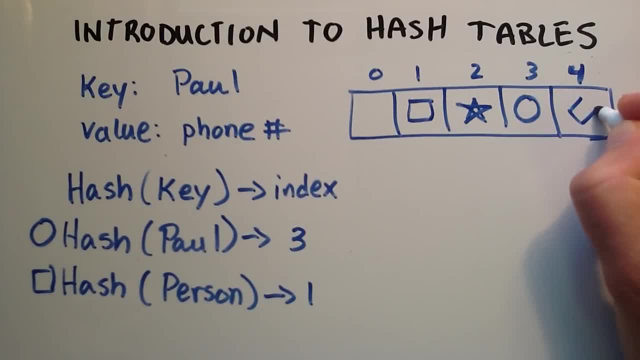 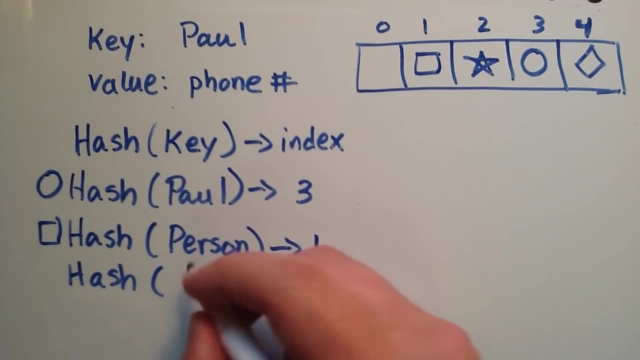 2. And maybe another one goes. they can be a diamond. I guess That will represent another person's name and phone number And we find that they go in index 4.. But what happens if we're wanting to add another person and we'll just put somebody? I don't know So. 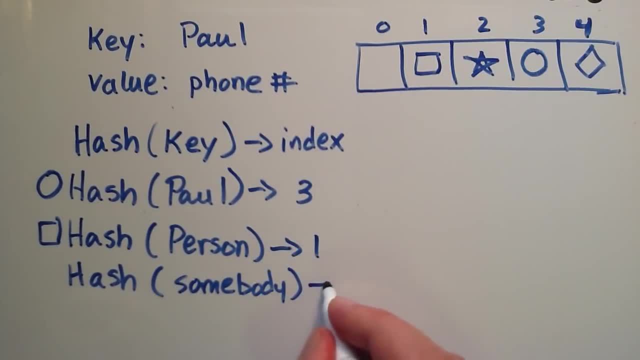 we're adding somebody else's number, And what if they? what if we find out that their hash value ends up being 3?? Well, we go and we look and we go, uh oh, there's already a name and phone number stored in index 3.. So there's a lot of different ways, to you know, to get. 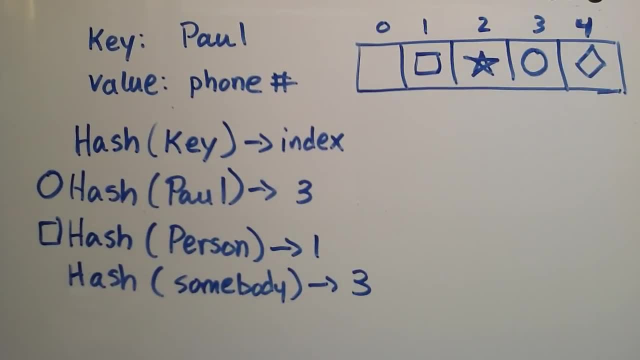 a to go about this to avoid a collision, And the way I'm going to implement this, when I code this in my videos in the next few tutorials, is I'm basically just going to create a link and create a basically just a linked list off of each one of these um indexes here. 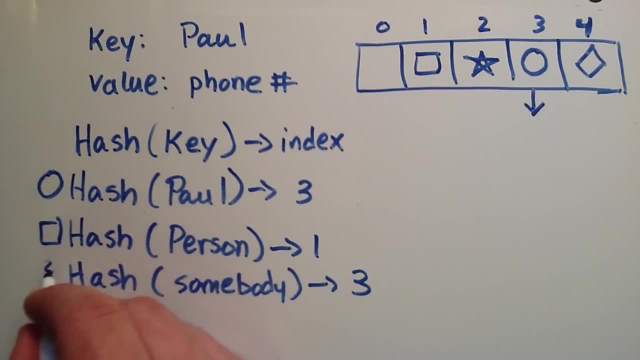 And so I don't know what shape we could use here. We could just do squiggly line or something like that. So what I would do here is I would just put squiggly line's name and phone number inside of this element here. So basically this is called chaining. So if we needed to, 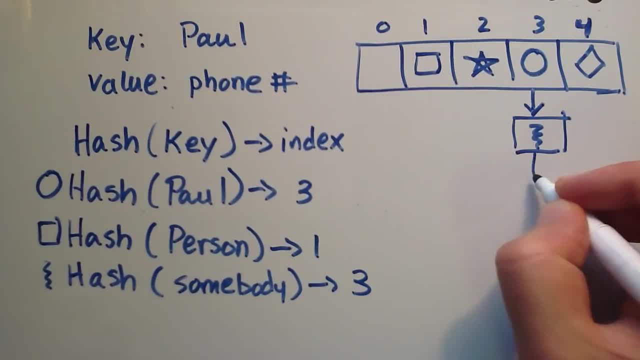 add more. let's say we got another one in index 3, we would just link that off of squiggly line's name and phone number And we could do sideways squiggly line That can represent that person's name or that, yeah, that person's name and phone number, And anyway I think. 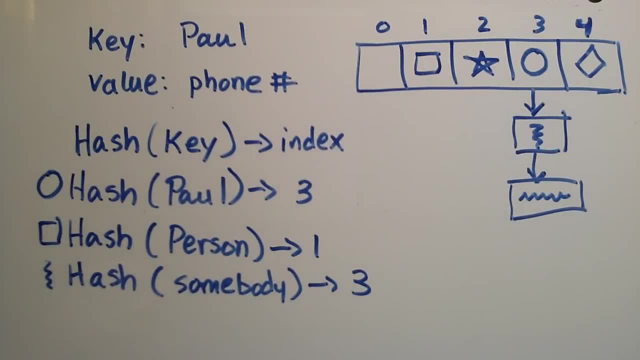 you guys get the point. So all these shapes just represent somebody else's name and phone number And if we end up with a collision then we basically are just going to link it off of that same element. So each one of these people's names and phone numbers they basically got. 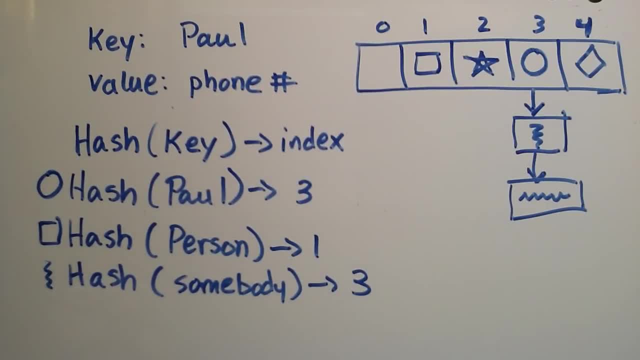 index 3.. And so the cool thing about this is if we get a whole bunch of names and phone numbers in here and then all of a sudden one day we want to go and look and we want to say, okay, where is you know, where is somebody's say you have the name of a person? 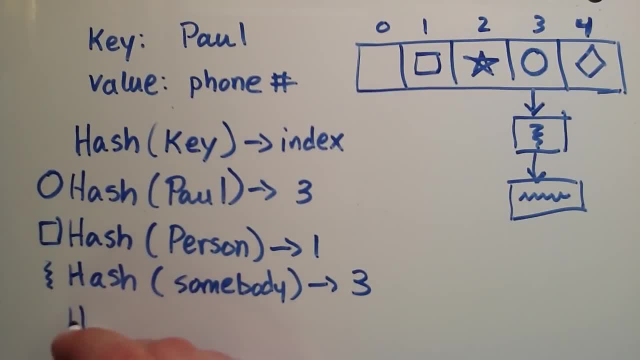 and you want to know what their phone number is. you basically just enter their key And the person has no access to those addresses that we have right now- can tell you there isn't. You can just type any number you want in there, but incorrectly you'll find it. design for. 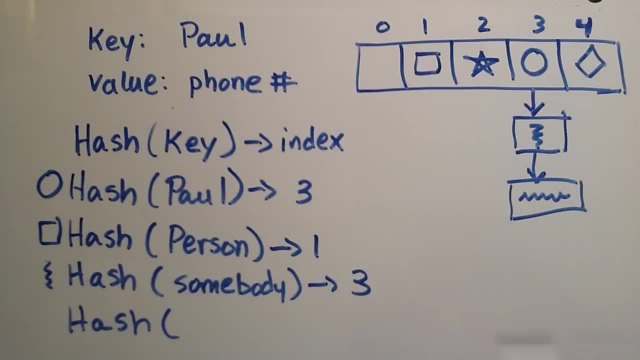 that person, wherever there is that person. Now, that would be super easy, but now we need people to input addresses that are like that one, Okay, And so if you can see here our home address and place each of the missing numbers one by one within this box, let's give that a Exactly. 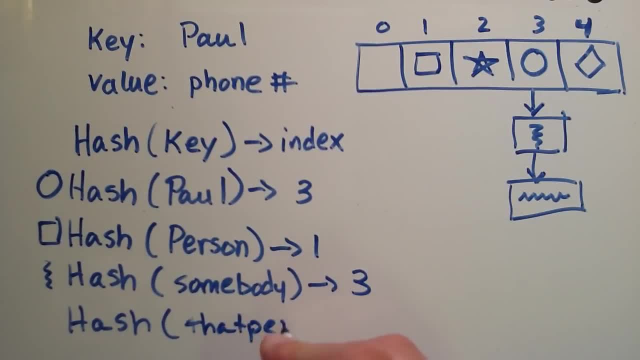 And so that's also doing brushcutting, and we just do: 🎵 име vaccine: panic shot 🎵. I'm using drug fashion And so if I was doing this thing, we actually just have to have simple numbers inside the hash function. 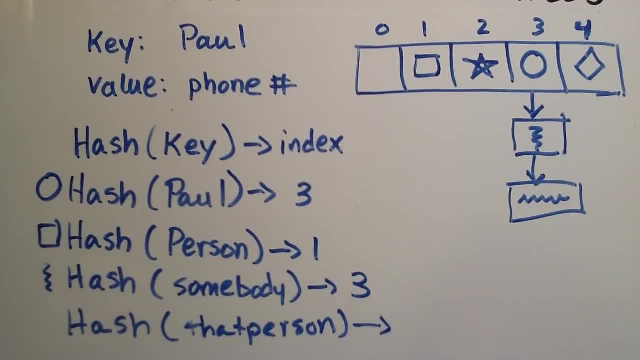 And so if there was like a gajillion different names and phone numbers, you could just do hash of you know whoever that person was- to basically spit out an index and it's going to tell you exactly where that person is located. and so it might be that that person- let's say we just got a whole bunch down here- 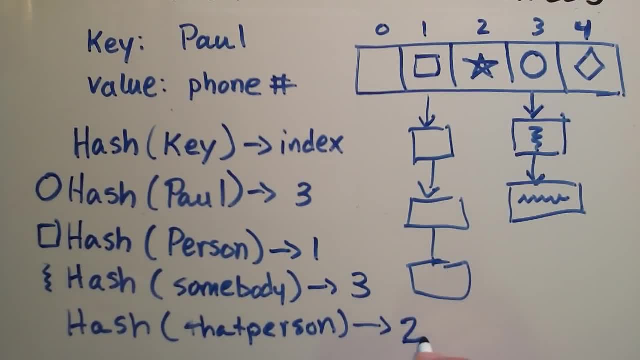 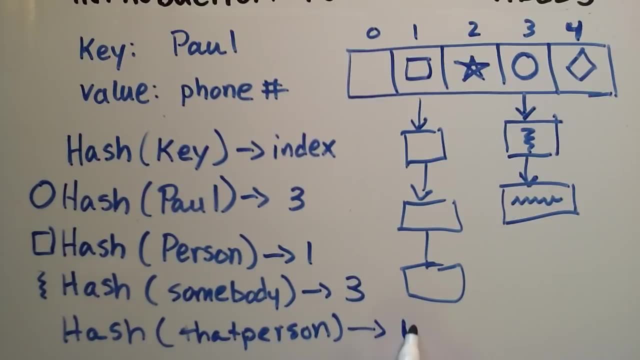 you know, it might be that that person is gets a hash value of two. so then what we do- or sorry, i meant to say one. so whatever person we're looking for might have a hash value of one. and then we know, even if this was like a million index units long, we know that we don't have to. 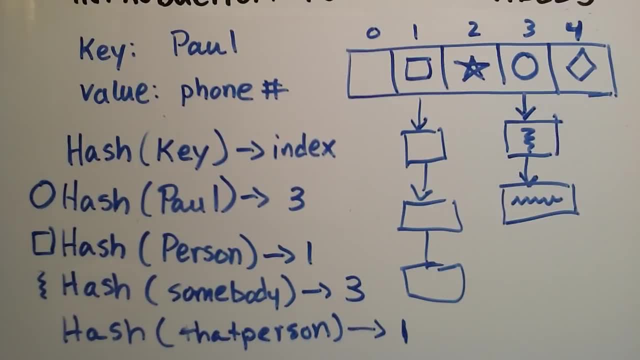 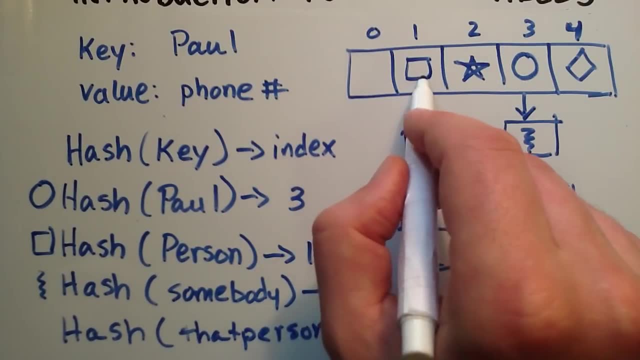 look in zero, two, three, four or all the way up to a million. we don't even have to look at those. our hash function tells us exactly which one to start at, and so then we would basically just start at this one, and if we had some chaining we could kind of go down the list and figure out.